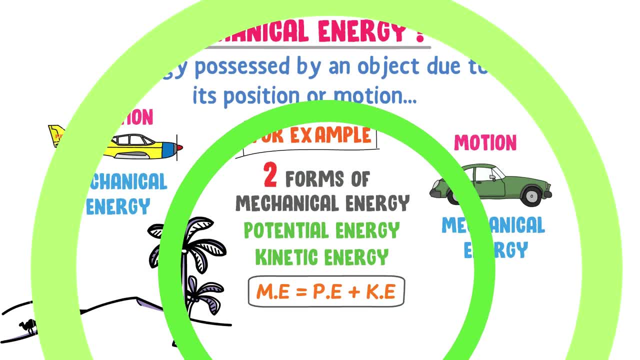 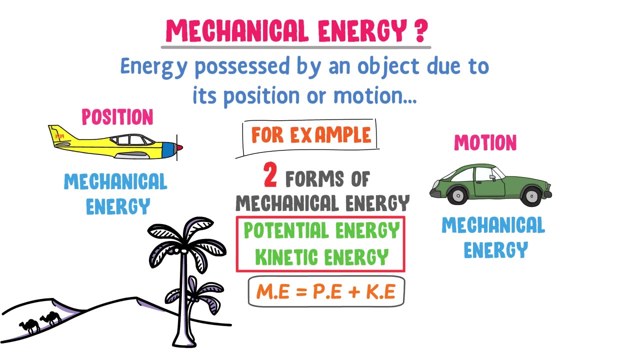 of potential energy and kinetic energy. Let me repeat it: Mechanical energy is equal to the sum of potential energy and kinetic energy. Thus, when you listen or read about potential energy and kinetic energy, always remember that they are the two different forms of mechanical energy. 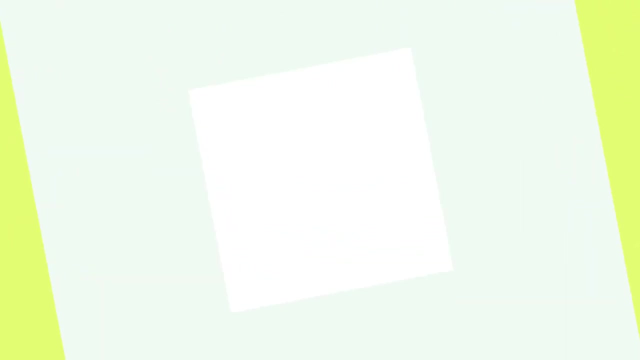 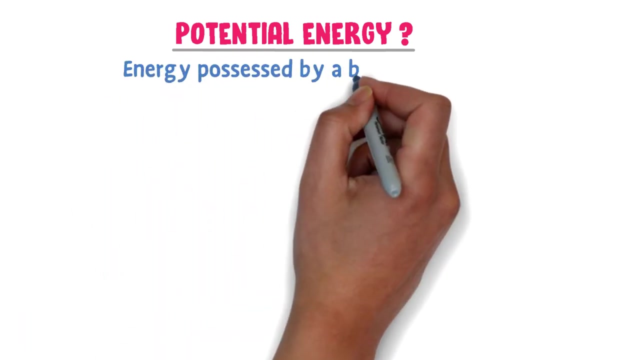 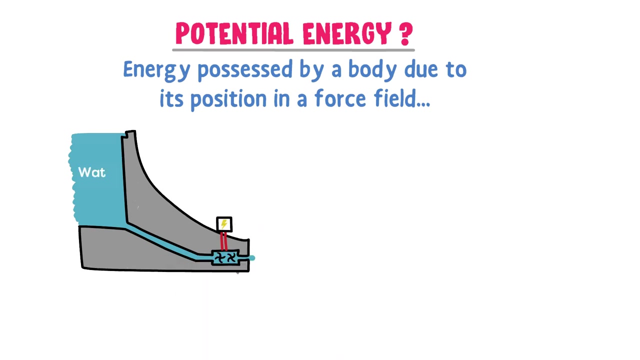 Now, what is potential energy? Well, potential energy is defined as energy possessed by a body due to its position in a force field. For example, water is stored and damps at a certain height. These stored water possess potential energy due to its height above the earth's surface. 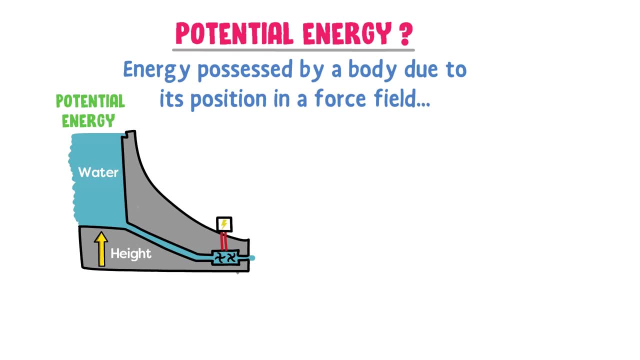 When these water falls, it is called energy. Now, what is potential energy? Well, potential energy refers to energy being composed of a container known as electron, and its energy actually contains the huge amount of hydrogen that's produced in a force field called electron. 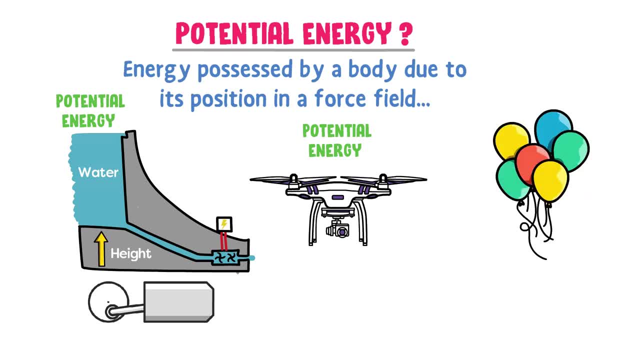 The photons which form electrons are located in the air. on Earth's surface They concentrate energy on ⁰. Premiumhe Z ⁰ Potential energy. To stepped up and up. they are called physical energy. left it above also possesses potential energy. 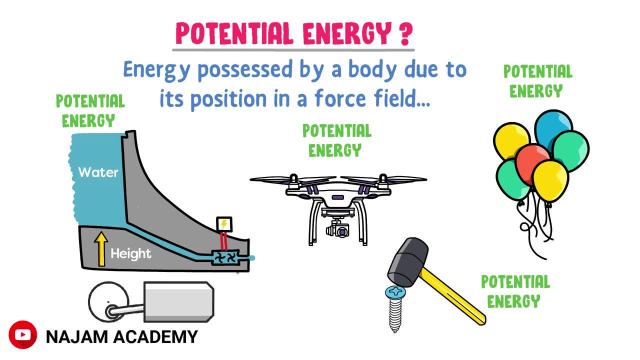 When you hit the nil potential energy of the hammer, do some sort of work on the nil and it sinks down into the world. Thus, remember that potential energy is the energy of an object due to its position, our height, and a force field like gravitational field. 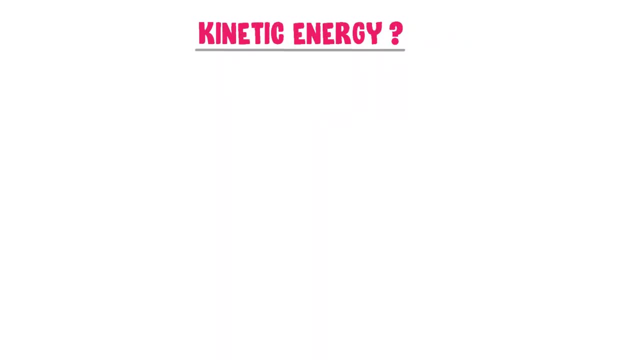 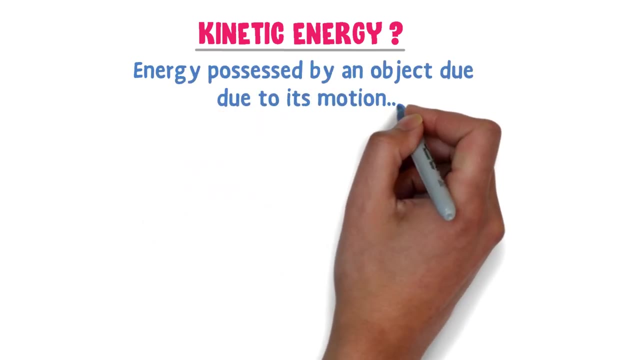 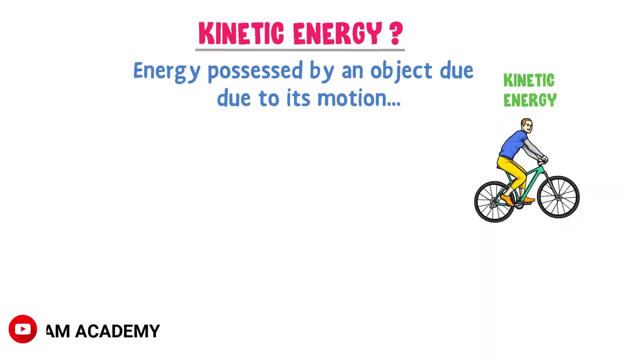 Now, what is kinetic energy? Well, kinetic energy is defined as energy possessed by an object due to its motion. For example, during cycling, you and your bicycle possesses kinetic energy due to motion. Secondly, in cricket match, when you hit a ball, the ball starts moving. 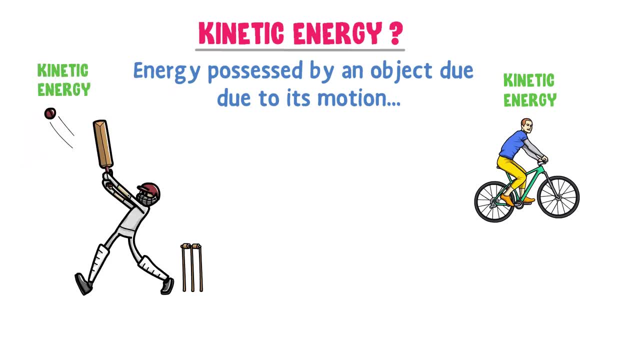 So this moving ball possesses kinetic energy. Thirdly, the hammer. The hands of a clock are constantly rotating around the fixed point. These hands of a clock also possesses kinetic energy due to their rotatory motion. Fourthly, when you kick a football, it starts moving. 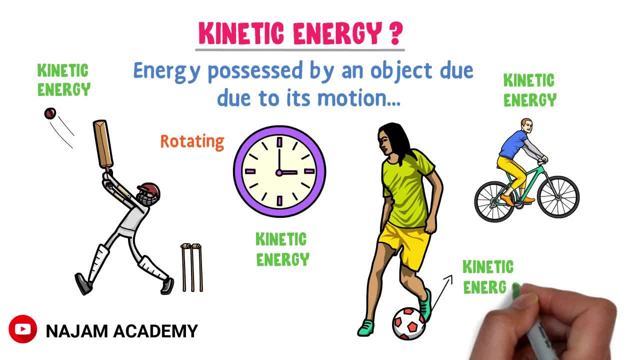 This moving football also possesses kinetic energy due to its motion. Thus, remember that if an object is moving, it possesses kinetic energy. Therefore, we say that energy possessed by an object due to its motion is called as kinetic energy.